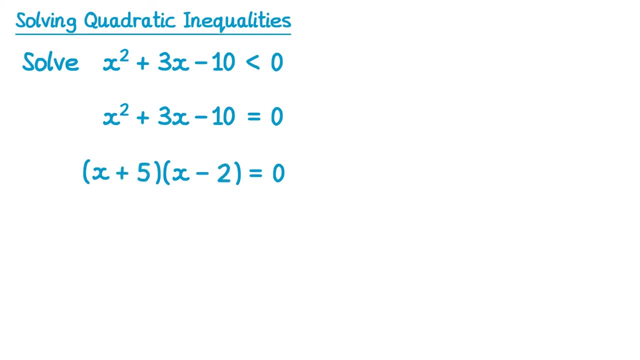 into two brackets. This one would be x plus 5 and x minus 2, and that would give solutions: x equals negative 5 and x equals positive 2.. These numbers here- negative 5 and positive 2, are known as critical values. We didn't want to solve the equation, though We wanted. 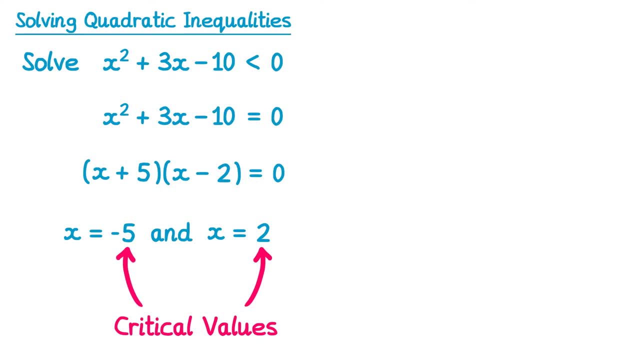 to solve when it was an inequality. To do this, we're going to draw the graph represented by the equation. So y equals x squared plus 3x minus 10.. We draw some axes. first of all, and we know that, since negative, 5 and 2 are critical values. 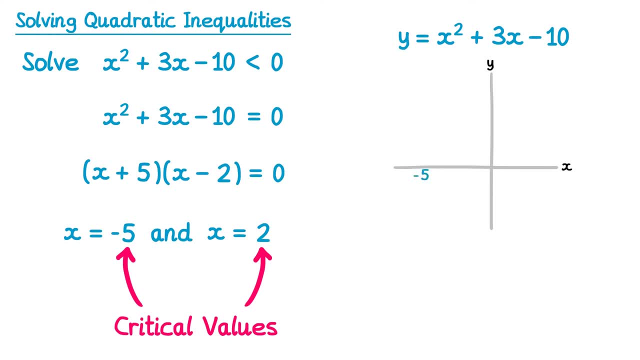 solutions to the equation. it must cross through these on the x-axis. We also know that quadratics like this make a nice u-type shape, so it would look something like this: Let's now consider our inequality again that we were trying to solve. If you substitute: 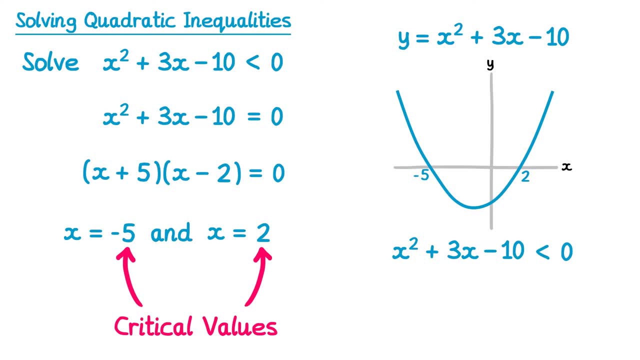 in the critical values you'll see that they're solutions because they give zero. So if we start with 2, 2 squared plus 3, lots of 2, take away 10.. Gives 4 plus 6, and 4 add 6, take 10, is zero. The same works for the other critical value. 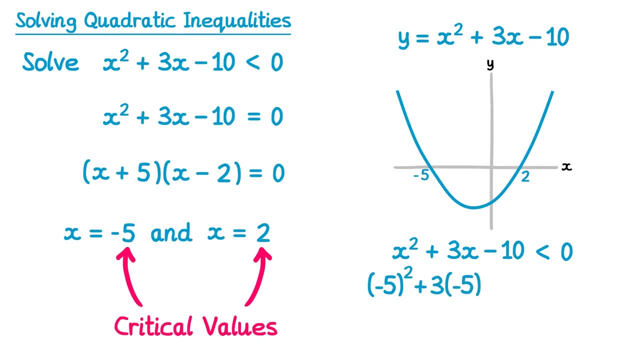 negative 5. Negative 5 squared plus 3. lots of negative 5, take away 10.. Gives 25 minus 15 and 25 take 15, take 10, again is zero. This shouldn't be surprising, since they were solutions to the equation, but we're. 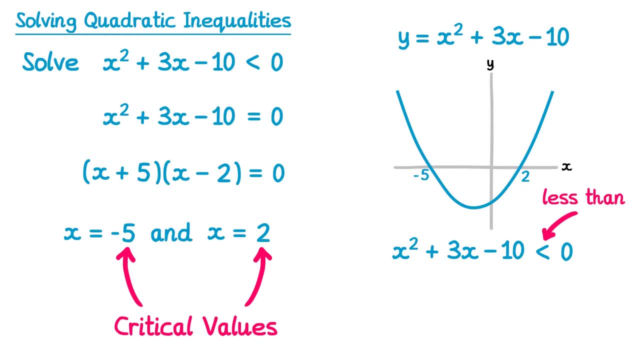 not interested in when it equals zero. We want to know when it's less than zero. So if we now look at the graph, you can see the graph is split into three parts: The first section- here, where the graph is above the axis. we then have this middle section. 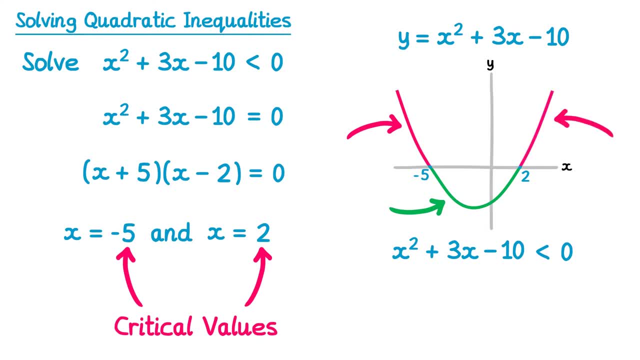 where it's below the axis, and this final section where it's above the axis. again, The two red sections are above the x-axis. This means that for those x values, the equation gave an answer that was greater than zero. The green section, however, is below the x-axis. 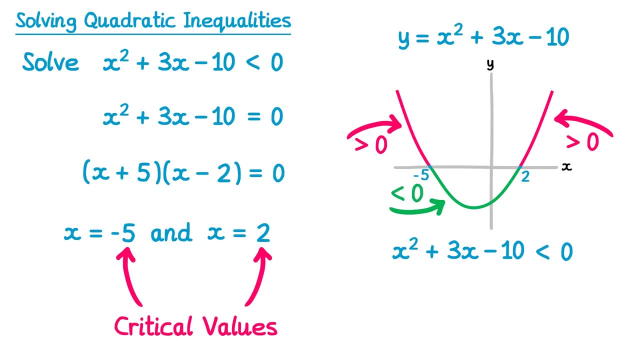 so for those x values, the equation gave an answer which was less than zero. Since our inequality asked for less than zero, we're interested in the green section of the graph To solve this inequality. then we want to know the x values that give this green section. 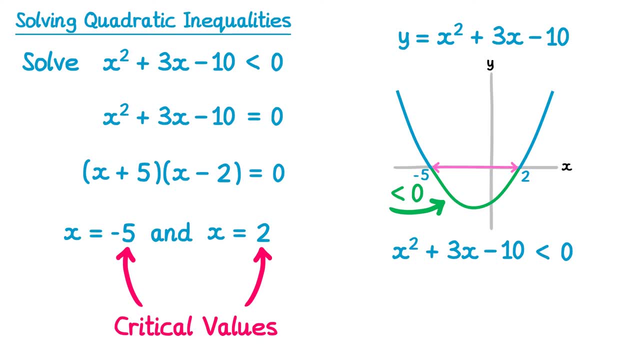 So that's all of the values marked here by the pink arrow. so in between negative 5 and 2.. We can write that down as an inequality: x is in between negative 5 and 2.. Notice, both of the inequality signs point to the left And that's the answer to this inequality. 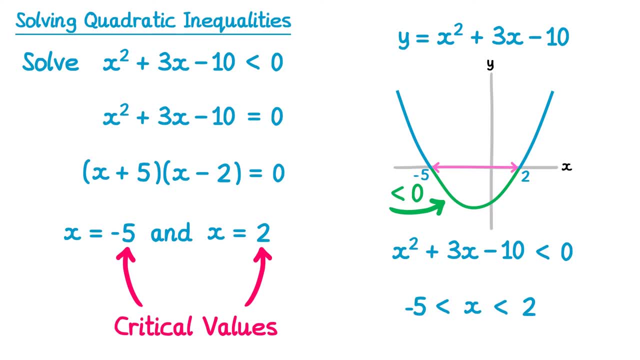 So what we did was, instead of solving the inequality, we first solved the equation to find the critical values. We now used to draw a sketch of the graph and then considered which section we were after. Once we had that section, we can write down the solution. Let's try a second one. 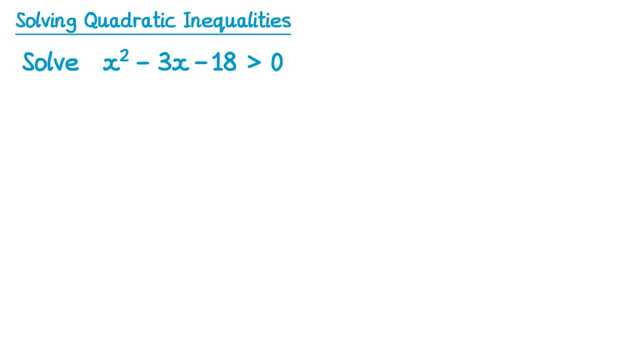 For this example, we have a greater than sign, but we'll still begin in the same way. We'll solve the equation. instead, To solve this equation, we can factorise The brackets. this time would be x plus 3, and x minus 6,, which gives solutions. x equals negative 3, and x. 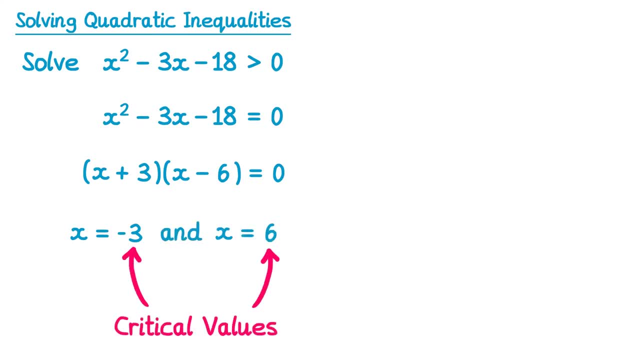 equals 6.. Remember, these are our critical values. So when we come to draw the graph, we know the graph will go through those critical values. so it must cross at negative 3, and it must cross at 6.. And again, this is a positive x. 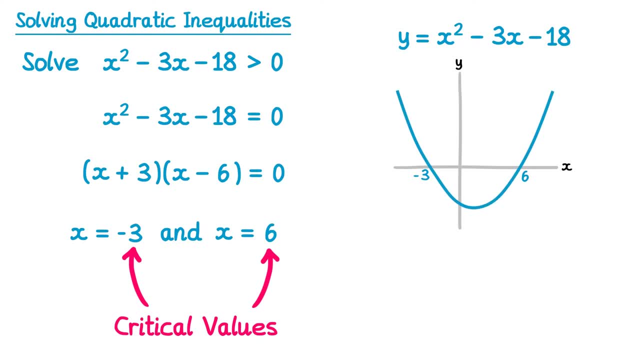 squared so it'll make a u type shape, something like this. We can now look back to the question: x squared minus 3x minus 18 is greater than 0.. Notice, this time it's a greater than sign. This means the section of the graph we're interested. 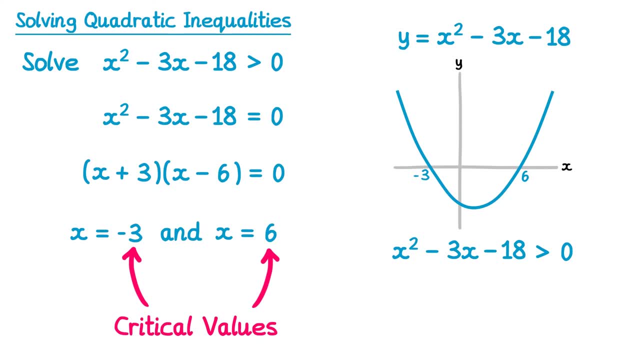 in is now above the x axis, So the section we want to look at is this section. So the x squared minus 3x is greater than 0.. Notice, the graph we're interested in is now above the x axis, So the section we want to look at is this section. The section we want to. 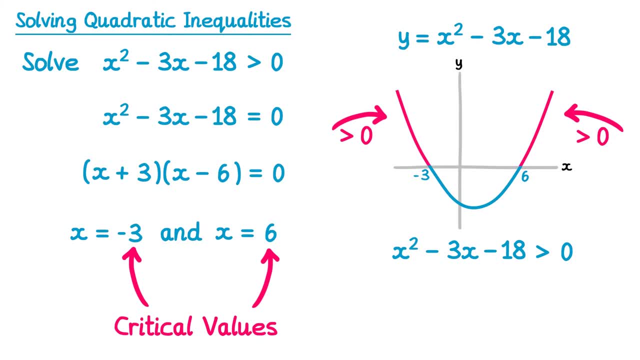 since it's greater than 0.. We then want to write down the corresponding x values that give us this section of the graph. This is now in two distinct parts. We have the part that is less than 3 here and the part that is greater than 6 here. 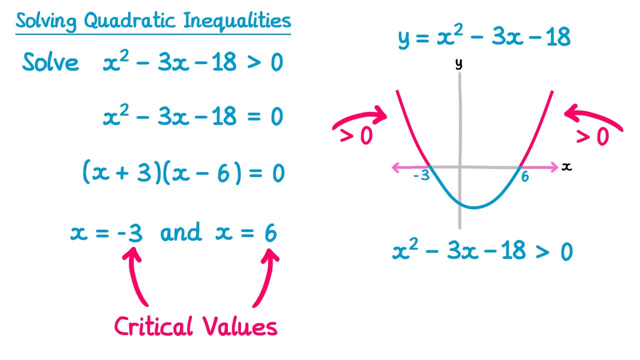 We can write these down as two separate inequalities: x is less than negative 3, or we have x is greater than 6.. When we solve a quadratic equation, we're used to writing the word and in between, because they're both acceptable solutions. This time we're going to write or, since you can't have a number that's less than. 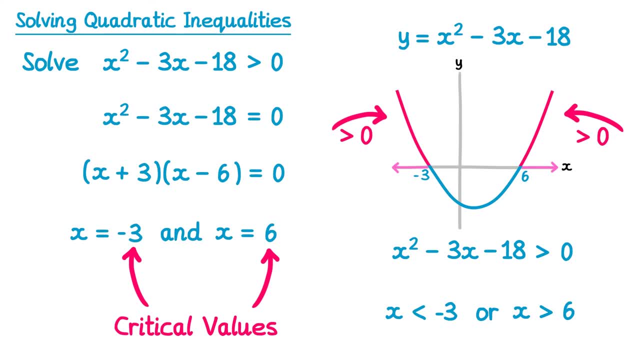 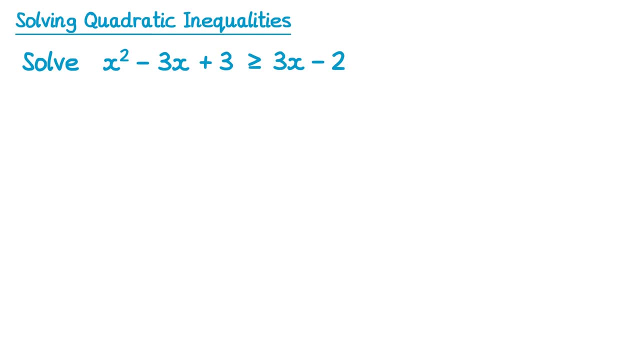 negative 3 and also greater than 6.. So when you have inequalities like this, we write an or instead. In this final example, there are two extra differences. Firstly, the symbol is now a greater than or equal to. This isn't going to change our approach, we just need to remember to write the extra. 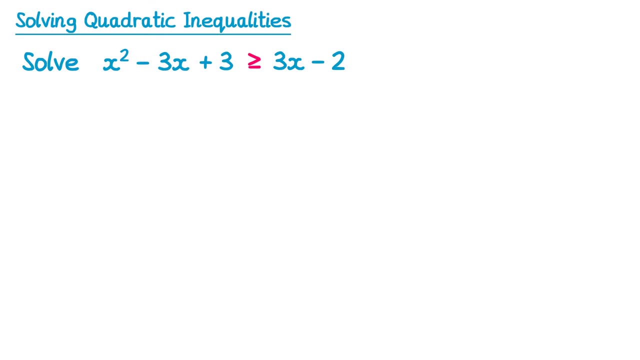 little line. This will be the same if it was less than or equal to. The second, though, will change. We have 3x minus 2 on the right hand side, where we're used to having 0. So we need to eliminate those terms before we begin To do this. we will subtract 3x and 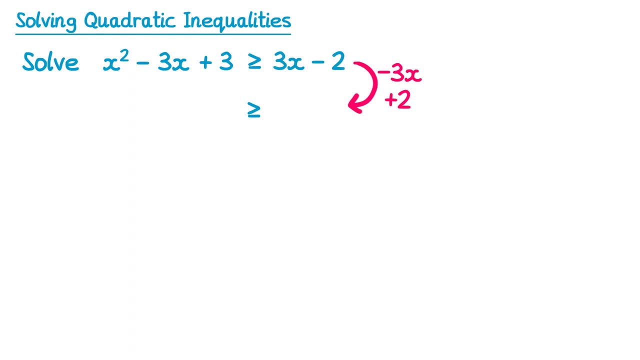 add 2 to the right hand side and then do the same to the left hand side. On the right hand side, this gives 0, since 3x- take away 3x- is 0 and negative 2- add 2 is 0.. On the left hand: 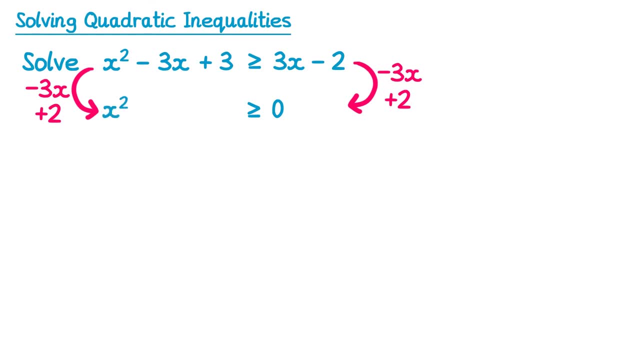 side, the x squared will remain unchanged. but then negative 3x. take away another 3x gives negative 6x, and 3 add 2 gives 5.. This inequality is now in the correct form. We can then look at solving the equation. So to factorise this one, you'd get x minus 1, x minus 5. 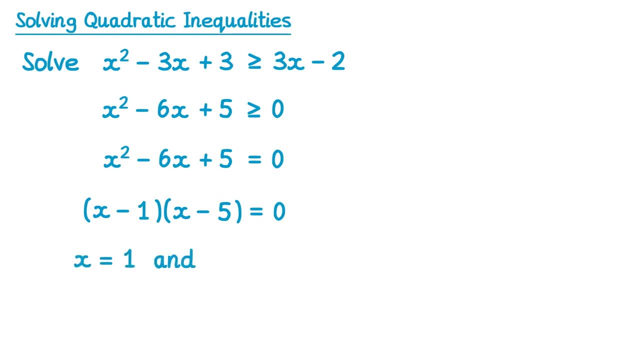 giving critical values: x equals 1 and x equals 5.. These critical values can then be plotted Ordinarily. at this point, we would draw the graph, and you can still do that. You'll still get to the solution. but I want to show you another method. 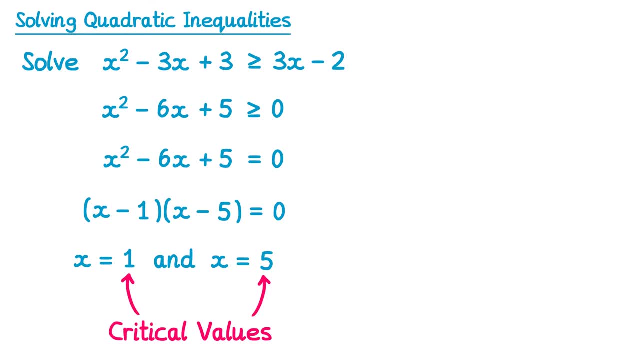 that some people prefer This method is case analysis. Instead of drawing the graph, we'll draw out just the x-axis and we'll plot on the critical values: x is 1, and x is 5.. These critical values split the x-axis into three distinct sections. The first section, 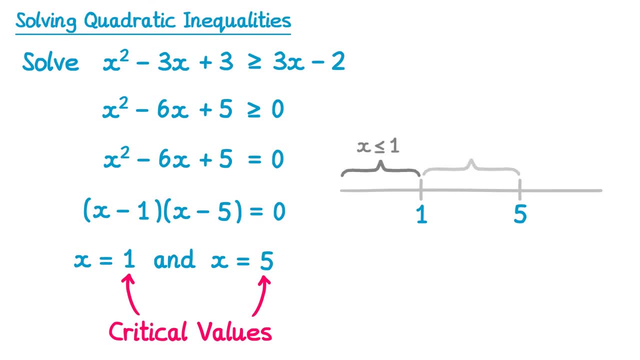 here on the left is when x is less than or equal to 1.. The next section in the middle is when x is in between 1 and 5 and the final section is when x is greater than or equal to 5.. Notice, I've used less than or equal to's and greater than or equal to's due. 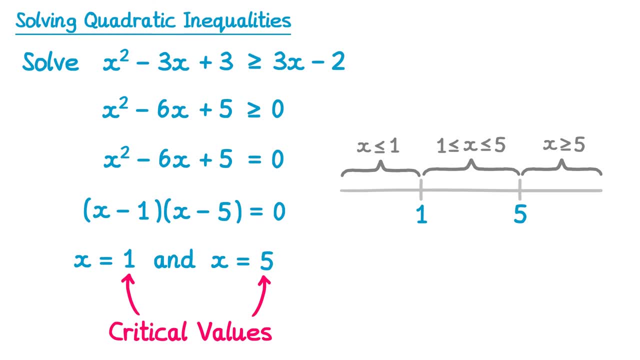 to the symbol in the question. I would next write down the inequality we're trying to solve And we'll go through each of these sections one at a time, checking if they're valid. So we'll start with the section on the left. x is less than or equal to 1.. We